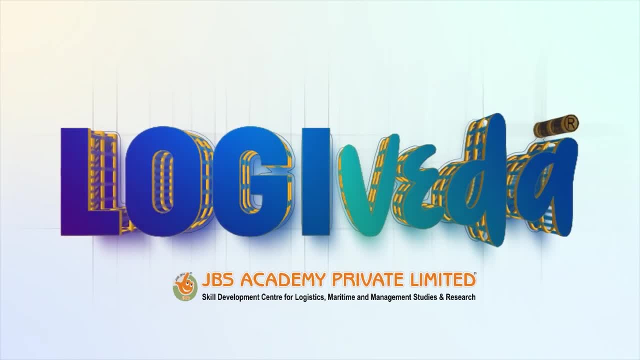 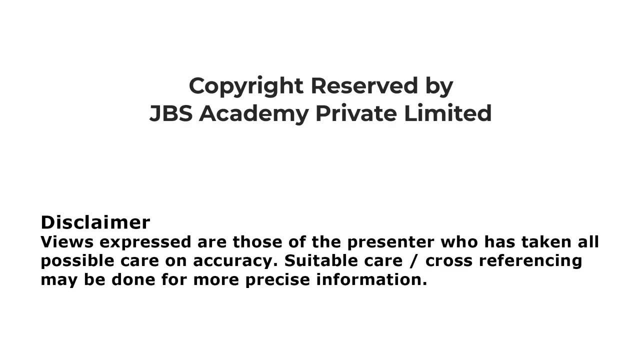 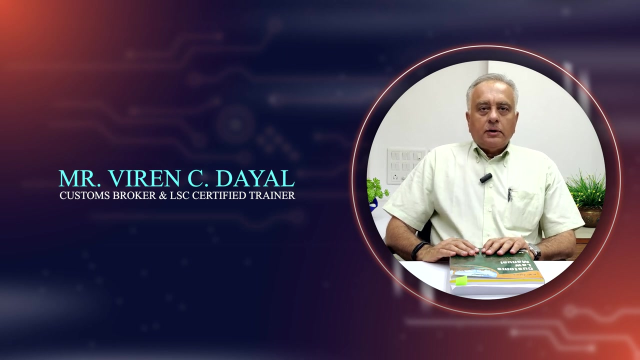 Hello everyone. my name is Viren Dayal. I am a custom broker and a logistic skill council certified trainer in customs law and applied rules and regulations. So today's topic I have chosen is on drawback. To give you a background note to drawback or to take back duties, taxes. 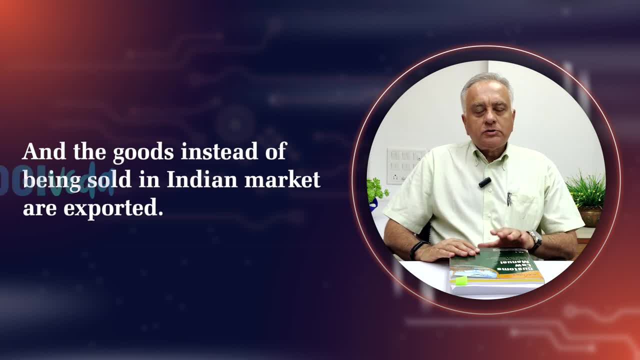 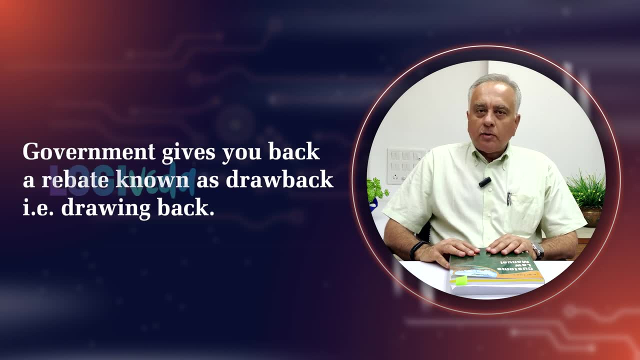 which are incurred in manufacturing of goods in India and the goods, instead of being sold in Indian market, are exported and therefore government gives you back a rebate, known as drawback. that is drawing back. The main purpose or the main aim of the government when we export goods is to export. 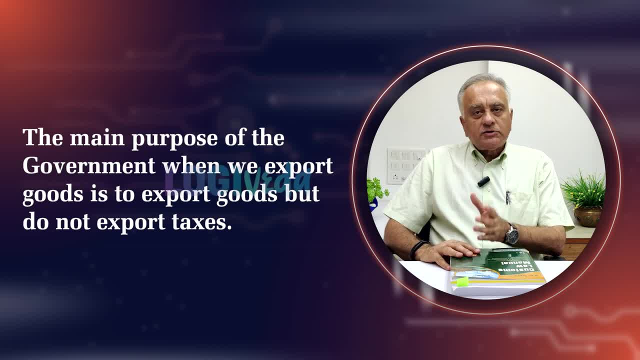 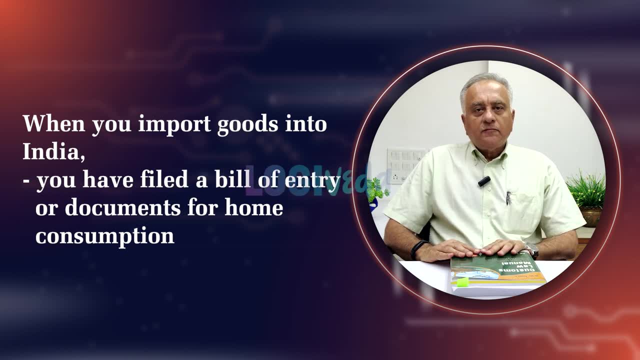 goods but do not export taxes. This is one of the concepts of drawback. The other concept is that when you import goods into India and you have filed a bill of entry or documents for home consumption, that means you pay the duty and you clear the goods from the customs area and then 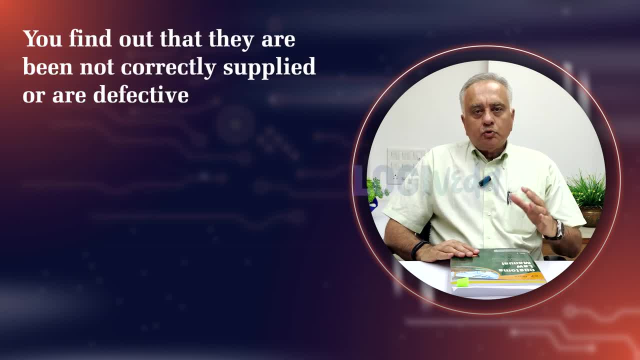 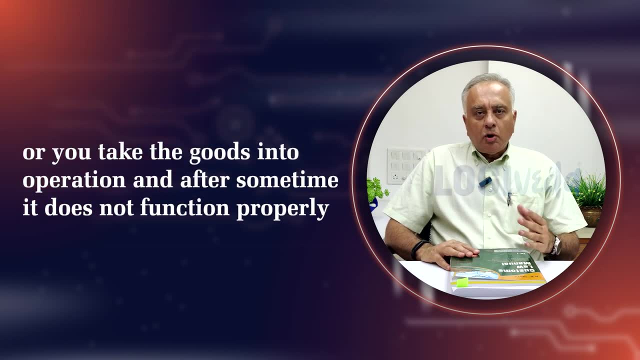 later on, when the goods reach your factory or your godown, you find out that they have been not correctly supplied, or maybe they are defective, or you take the goods into operation, like a printing press or maybe a shuttlerless machine, shuttlerless loom weaving machine, and so on, and after some, 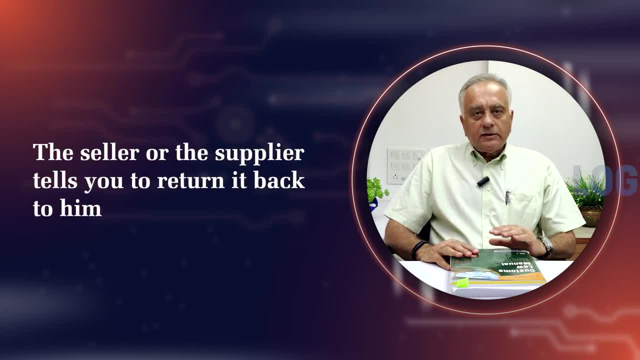 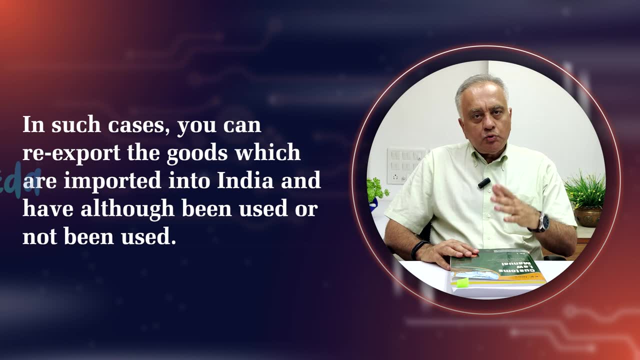 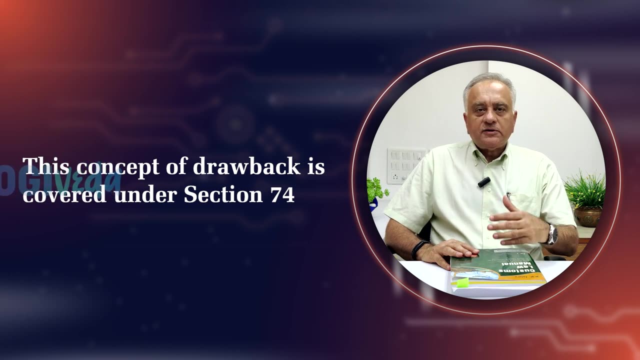 time the goods function properly and the seller or the supplier tells you to return it back to him. In such cases you can re-export the goods which are imported into India and have, although been used or not been used, and this concept of drawback is covered under section 74.. So section 74 is the 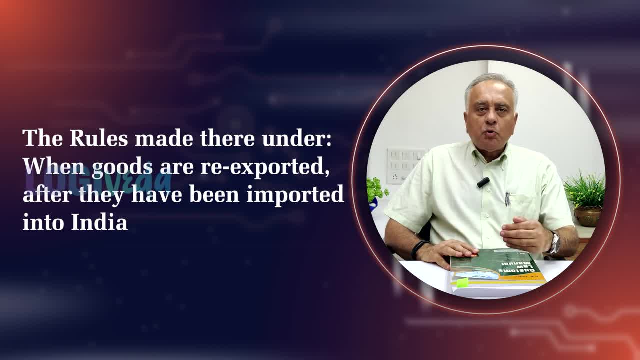 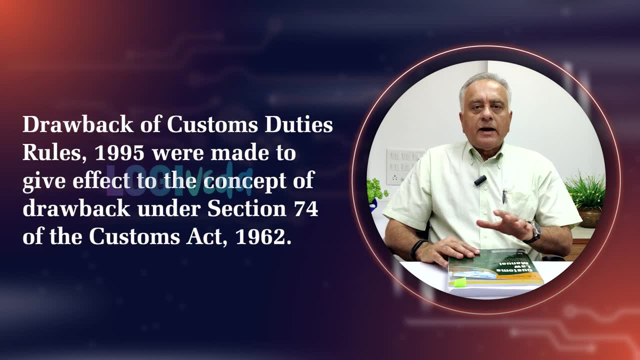 first section I'll be talking about and the rules made there under when goods are re-exported after they have been imported into India. Re-export of imported goods, drawback of customs duties. rules 1995 were made to give effect to the concept of drawback under section 74 of the customs act 1962. 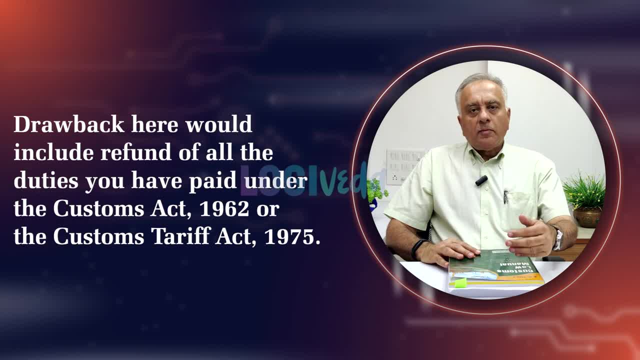 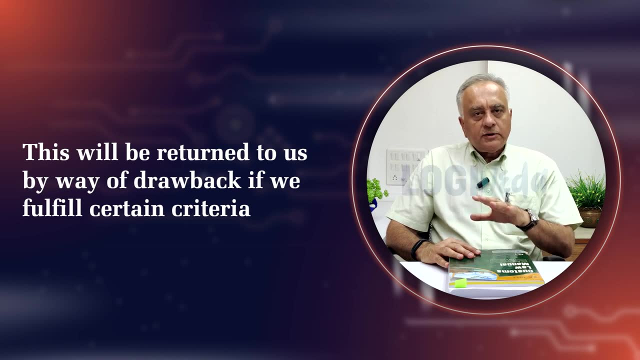 The scope of the section and the rules is that drawback here would include refund of all the duties you have paid under the customs act 1962 or the customs tariff act 1975. This will be returned to us by way of drawback if we fulfill certain criteria, namely the goods are imported into India. 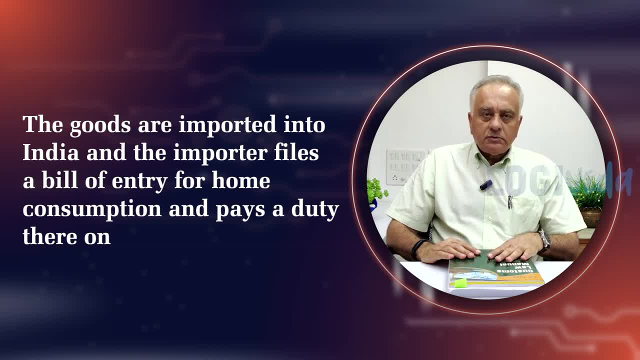 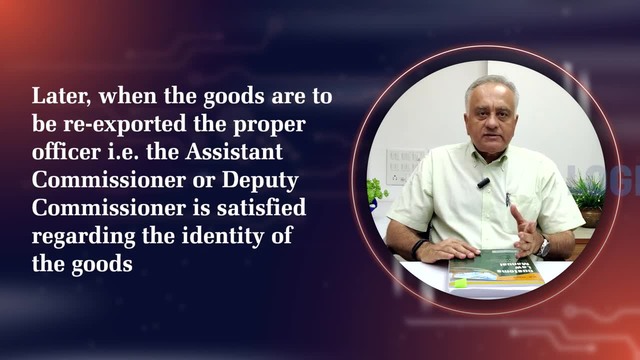 and the importer will pay the cost of the goods and the importer will pay the cost of the goods. Files are below entry for home consumption and pays are duty thereon. Later on, when the goods are to be re-exported, the proper officer, that is the ACO. the DC is satisfied regarding the identity. 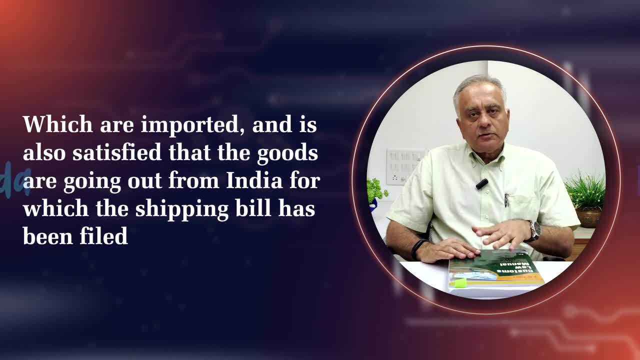 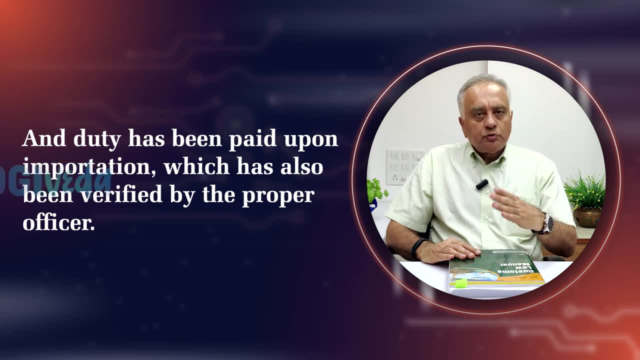 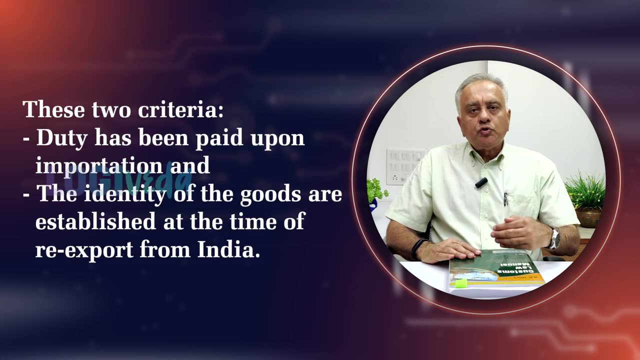 of the goods which are imported and is also satisfied that the goods are going out from India, for which a shipping bill has been filed, and duty has been paid upon importation, which has also been verified by the proper officer. So these two criteria, the duty has been paid upon importation and the identity of the goods, are 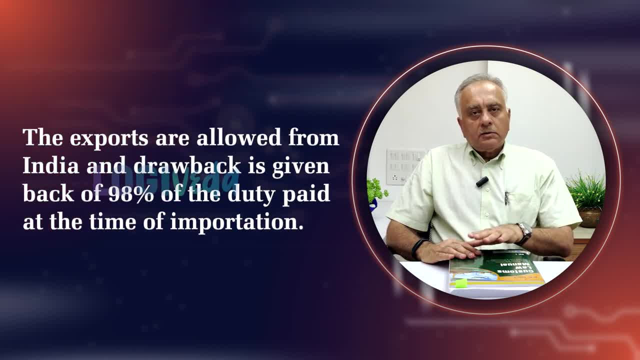 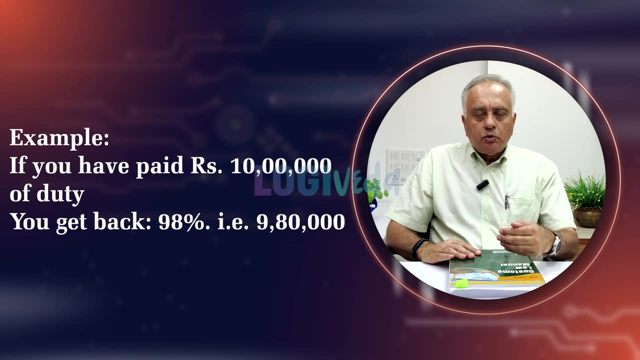 established at the time of re-export from India. The exports are allowed from India and drawback is given back of 98% of the duty paid at the time of importation. As an example, if you have paid 10 lakh rupees of duty, you get back 98%, that is 9,80,000, and 2% duty is generally. 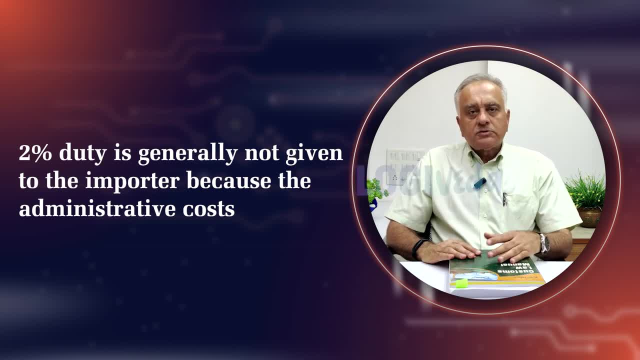 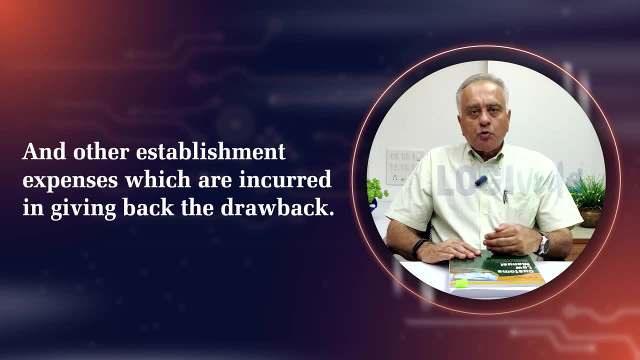 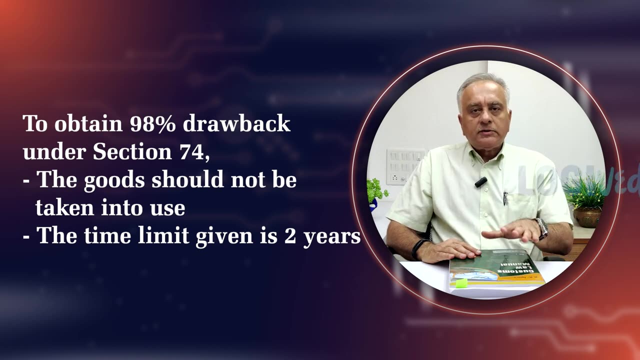 not given to the importer because the administrative costs and other establishment expenses which are incurred in giving back the drawback. Also, it's important to know that to obtain 98% drawback under section 74 the goods should not be taken into use and the time limit given is. 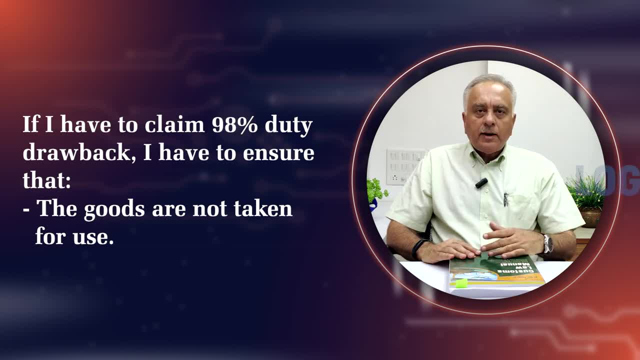 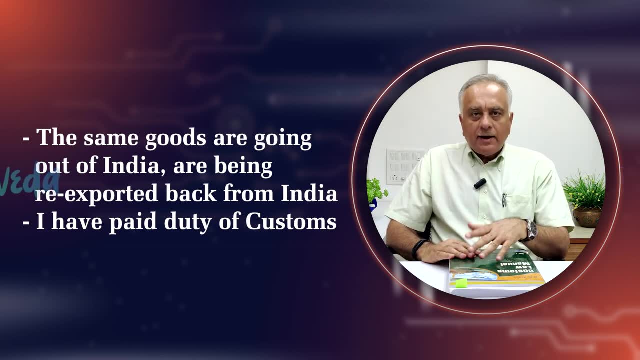 two years and therefore, if I have to claim 98% duty drawback, I have to ensure that the goods are not taken for use. the same goods are going out of India, are being re-exported back from India and I've paid a duty of customs and I shall get back 98%. 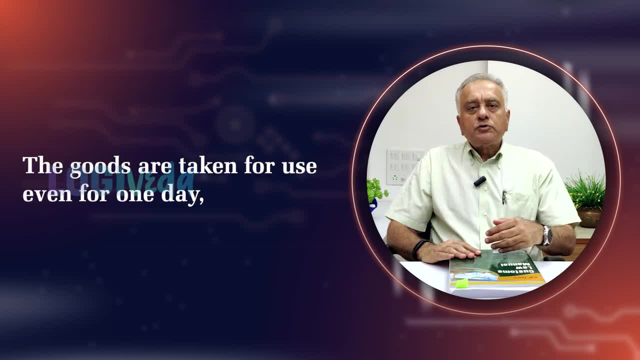 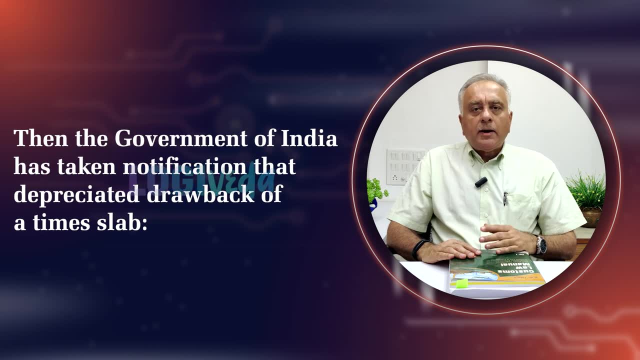 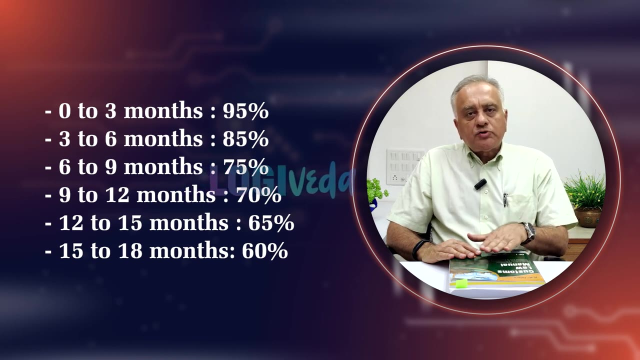 as a duty. drawback In the second scenario, where I've taken the goods for use even for one day, then the government of India has taken a notification that I will get depreciated drawback of a time slab of 0 to 3 months: I get 95%. if I use the goods from 3 to 6 months, I get 85%. 6 to 9 months, then I get 75%, 9 to 12 months 70%, 12 to 15 months and 15 to 18 months 60%. So depending upon how much goods have taken for use, I will get a depreciated drawback, and after 18 months there is no provision for any refund. 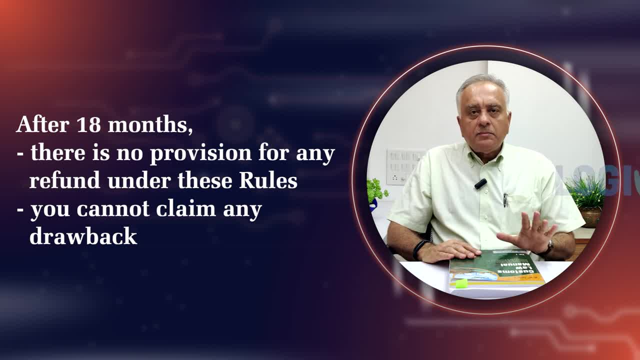 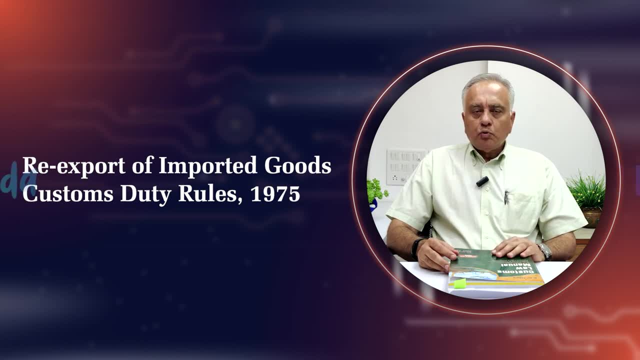 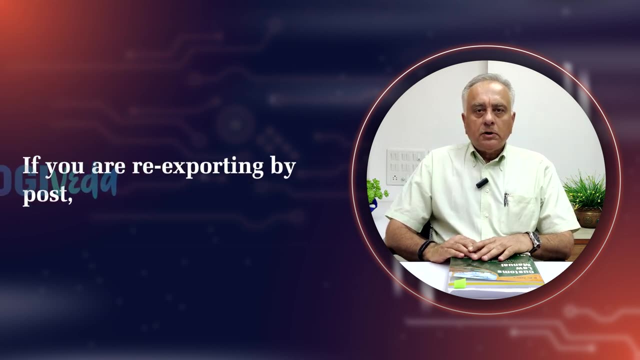 under these rules and therefore after 18 months you cannot claim any drawback. Re-export of imported goods: customs duty rules 1975 also stipulate certain rules that if you are re-exporting by post, then within how many days and what is the procedure to be.